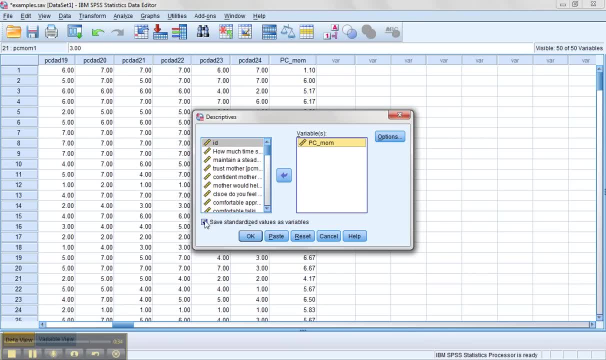 variable PCMom, and I'm going to check that box to say Save Standardized and notice it underlines the z for you z values. Save Standardized Values as Variables and then I'm going to go ahead and hit OK, Looks lovely, I can definitely. 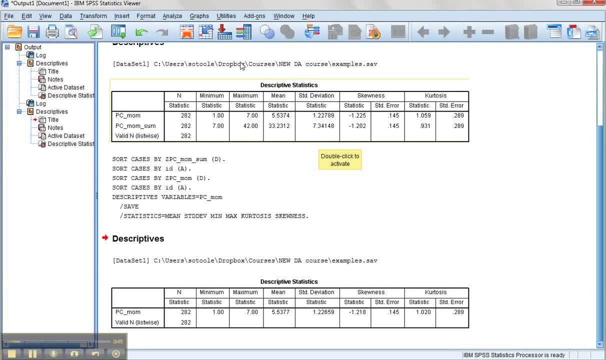 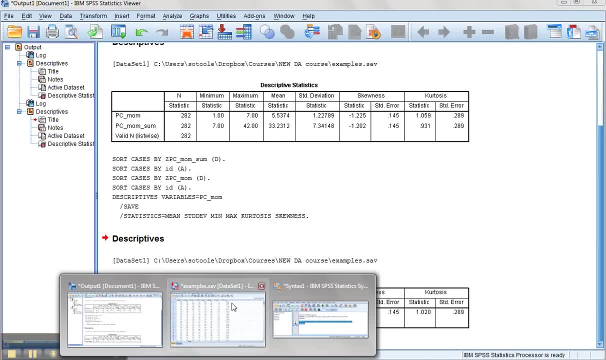 see it's a little bit skewed to the negative end. We have a little bit of kurtosis going on. so let's go back and check and see how those z-scores are going to be. Let's see how those z-scores look. We can just pop back to our data set. We can then right-click on it. I can see one already. We can hit Sort Ascending. 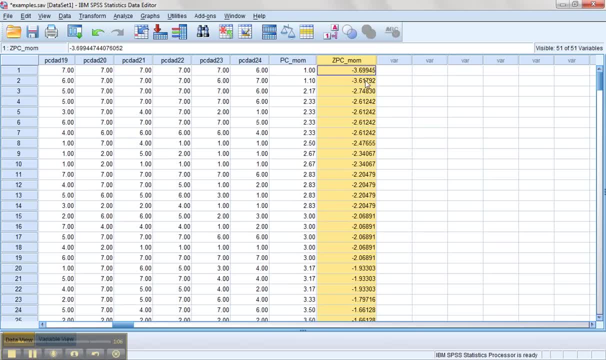 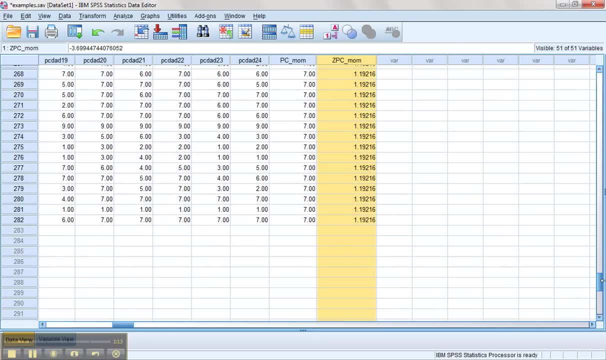 There we go. So our two negative outliers are at the top. Let's go ahead and check the other end of the distribution by just going ahead and scrolling down and down there. our highest z-score on the positive end is a 1.19.. Definitely not an. 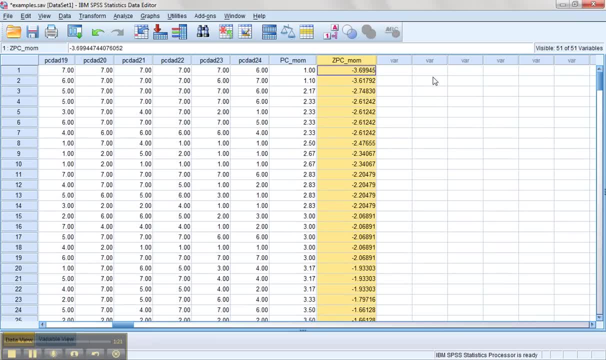 outlier. These, however, on the negative end, are both outliers. Anything greater than a 3.29 is an absolute outlier. So this one's an outlier and that one's an outlier, And I can see. luckily it's right next to the variable I'm looking at. I can see that the values on PCMom. 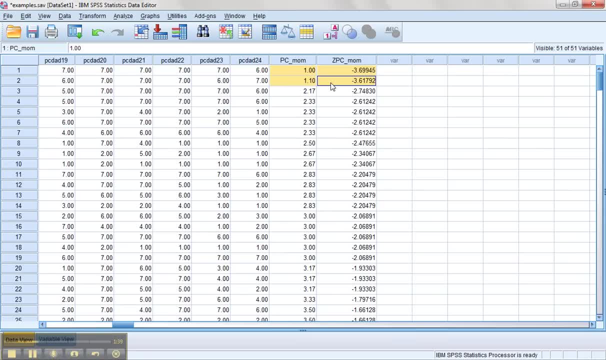 that are problematic are 1.0 and 1.10.. So anything actually less than a 2 would work in this case, because greater than a 2 would be our next value. You just need to pick any value between these if we want to go ahead and use it as missing. 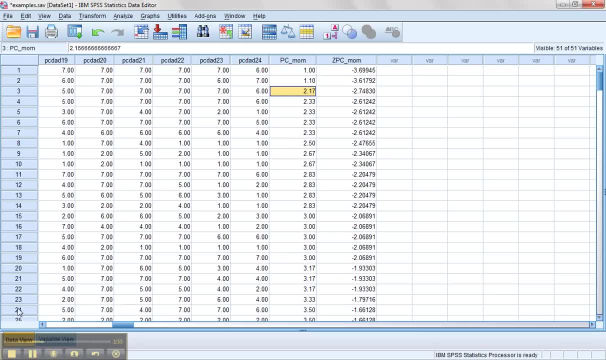 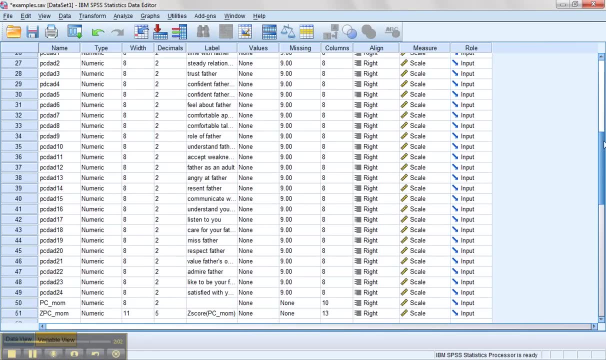 data and put that into the variable view. So let's go ahead and try that. I'm going to click on, we'll see variable view And I'm going to come down here and I want to make sure I'm setting the. 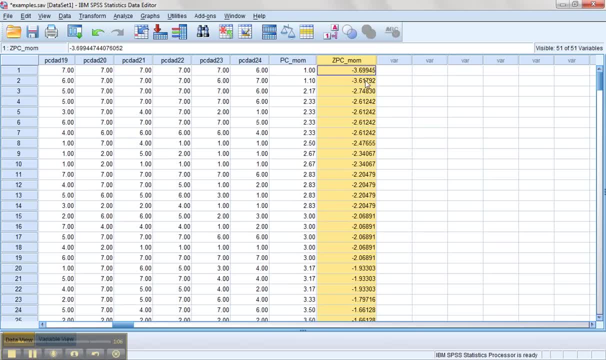 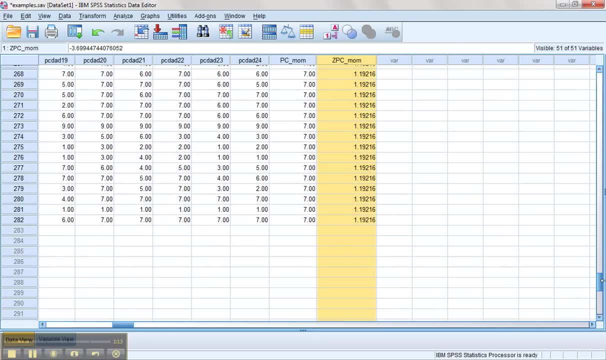 There we go. So our two negative outliers are at the top. Let's go ahead and check the other end of the distribution by just going ahead and scrolling down And down. there, our highest z-score on the positive end is a 1.19.. Definitely not an. 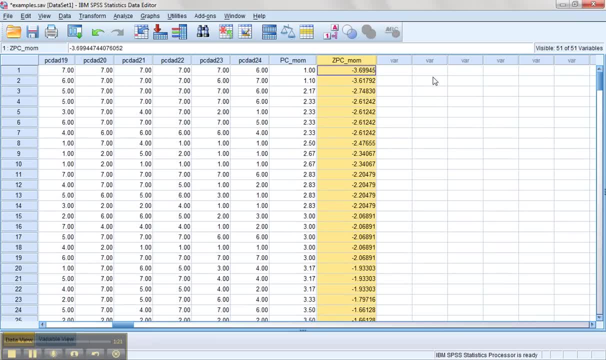 outlier. These, however, on the negative end, are both outliers. Anything greater than a 3.29 is an absolute outlier. So this one's an outlier and that one's an outlier, And I can see. luckily it's right next to the variable I'm looking at. I can see that the values on PCMom. 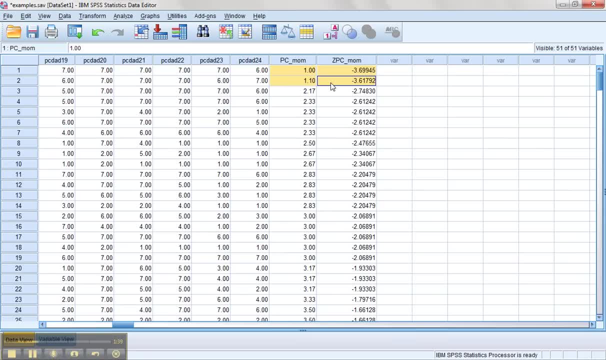 that are problematic are 1.0 and 1.10.. So anything actually less than a 2 would work in this case, because greater than a 2 would be our next value. You just need to pick any value between these if we want to go ahead and use it as missing. 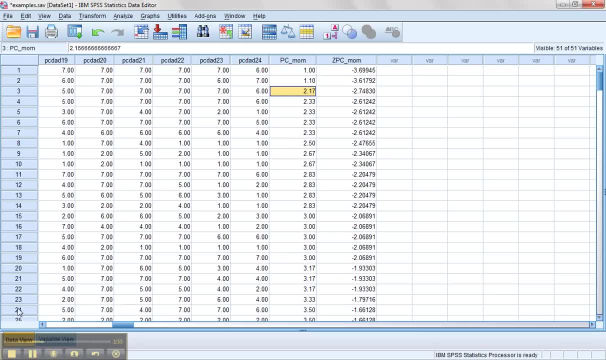 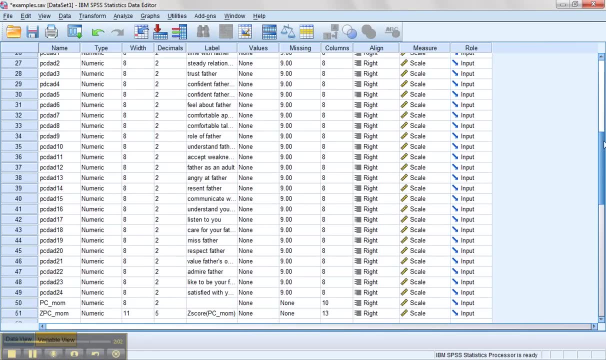 data and put that into the variable view. So let's go ahead and try that. I'm going to click on, we'll see variable view And I'm going to come down here and I want to make sure I'm setting the. 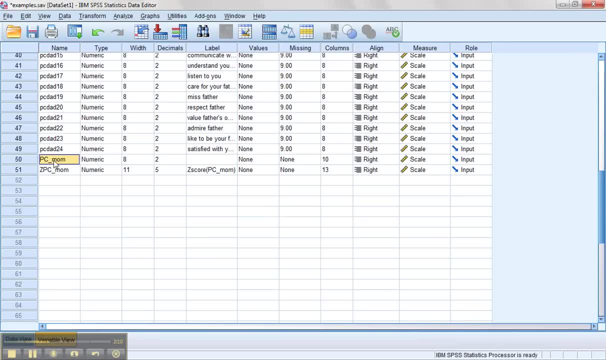 variables, the missing values for the actual variable, so in this case PCMom, not for the z-scores on PCMom. So I'm going to go in here and I can use the range, And the range at this point is anything from zero to zero. 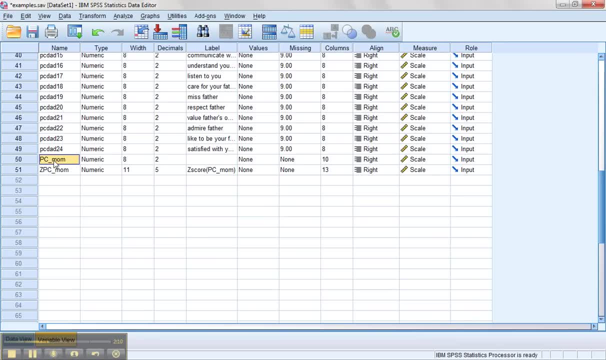 variables, the missing values for the actual variable, so in this case PCMom, not for the z-scores on PCMom. So I'm going to go in here and I can use the range, and the range at this point is anything from zero. 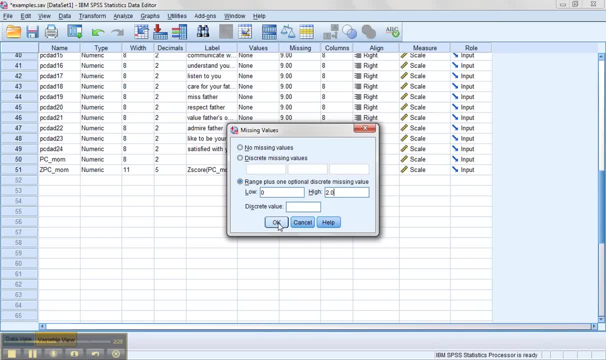 to 2.0, it will consider missing And I can go ahead and click on OK at that point. If we also had some missing values that are just you know, one of the usual ones we use to just mark missing values is 9.0.. So if we had that missing values, 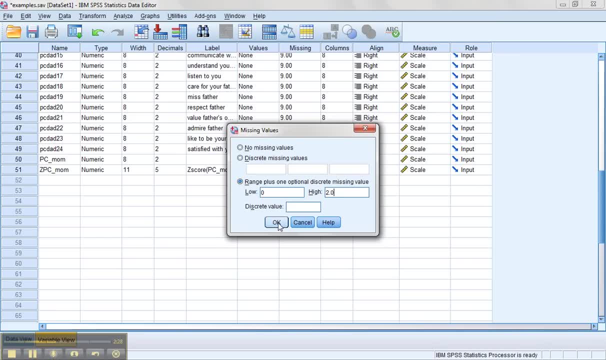 And if we go back to 2.0, it will consider missing And I can go ahead and click on OK at that point. If we also had some missing values that are just one of the usual ones we use to just mark missing values is 9.0.. So if we had that missing, 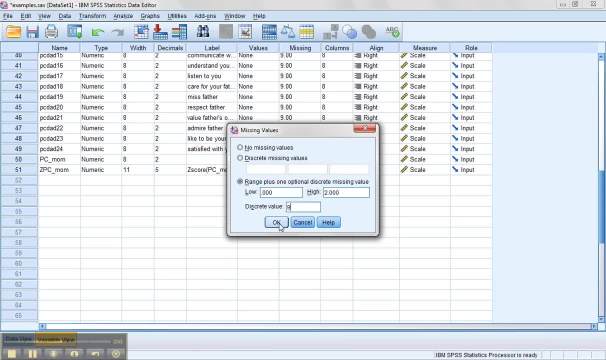 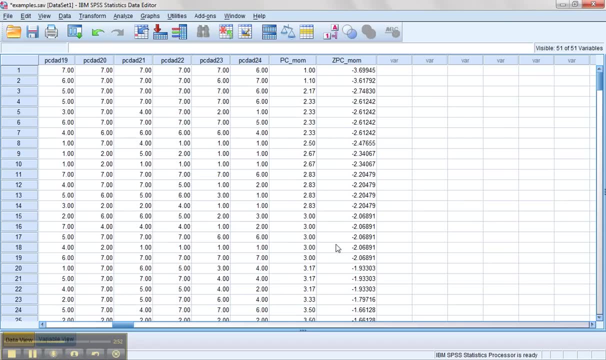 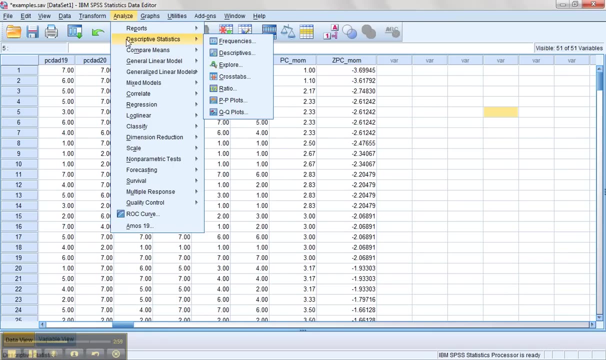 values of 9, we could go ahead and mark that as that extra discrete missing value and hit OK. Then we can go ahead and hop back to our data And it preserves the data. It's still here, but you'll notice that if we reanalyze that, we'll go ahead. 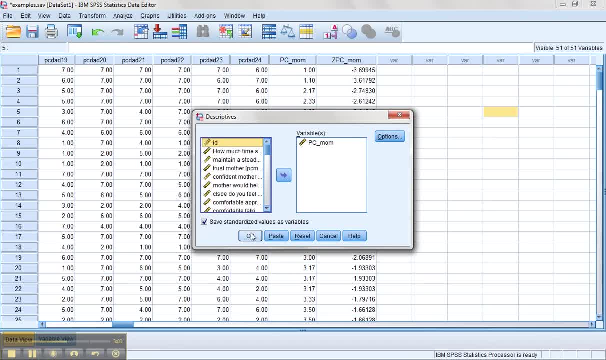 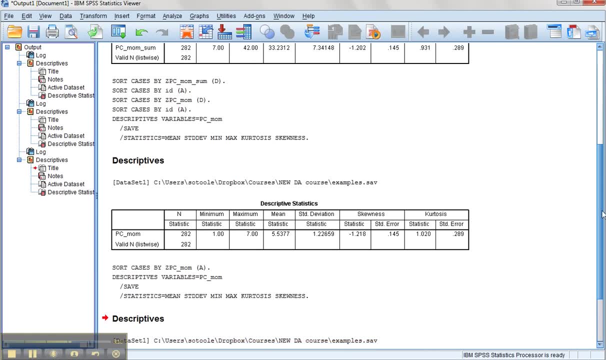 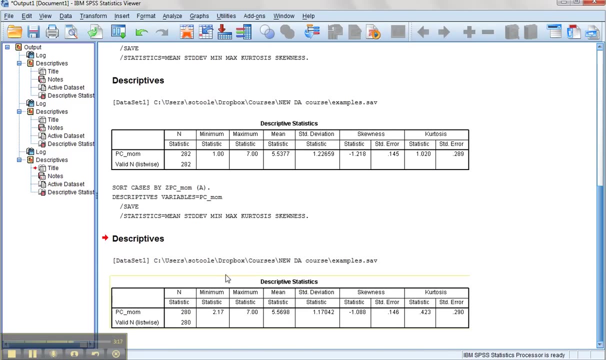 and grab some descriptives again, you will notice that our originally, our originally, our original values on that were from 1 to 7, with a mean of 5.53.. Now we've taken that missing value out and we can tell that it worked, because 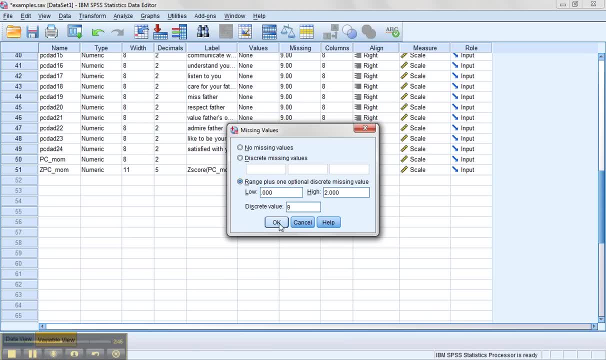 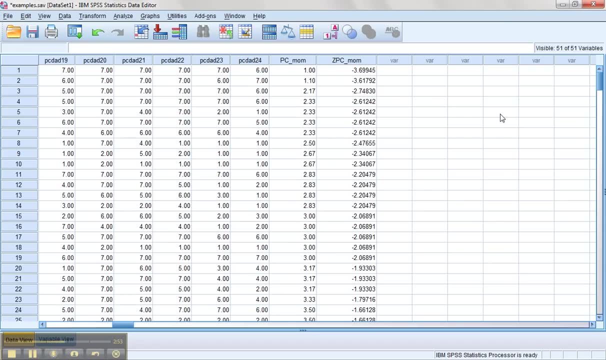 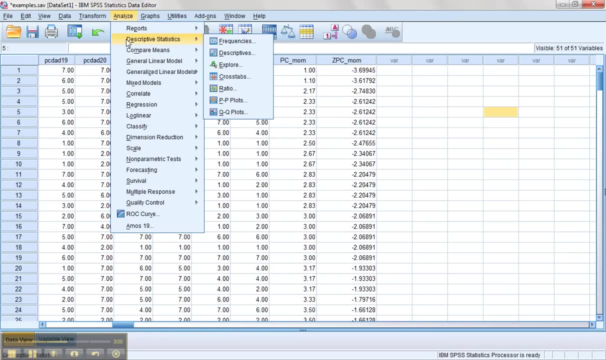 of 9, we could go ahead and mark that as that extra discrete missing value and hit OK. Then we can go ahead and hop back to our data And it preserves the data. It's still here, but you'll notice that if we reanalyze that, we'll go ahead. 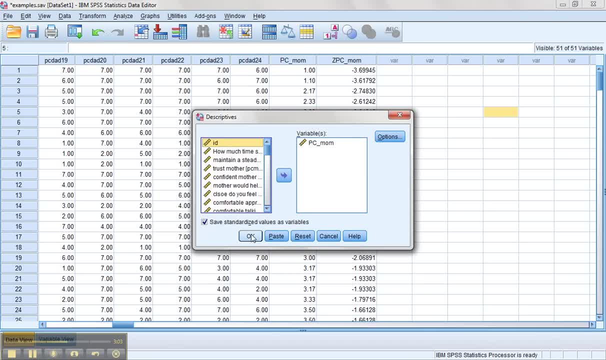 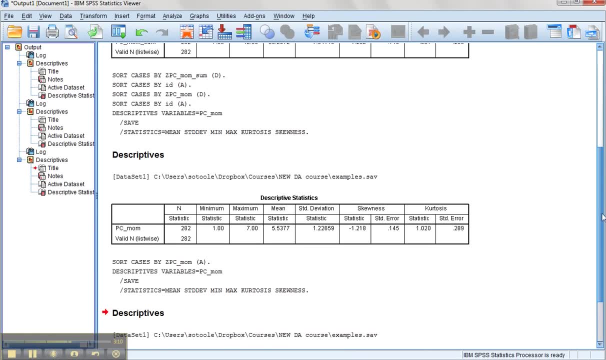 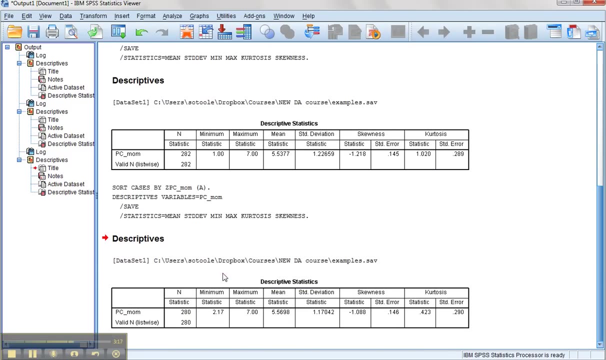 and grab some descriptives again, You will notice that our originally, our originally, our original values on that were from 1 to 7, with a mean of 5.53.. Now we've taken that missing value out and we can tell that it worked, because 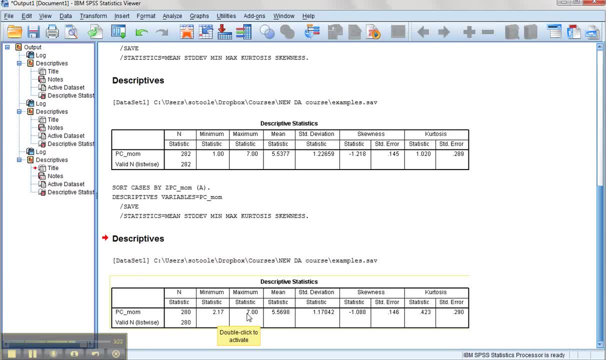 now our minimum is 2.17 and our maximum is 7.. And that was the first, that 2.17 was the first value that was not an outlier. So we cut it correctly and our skewness improved, but only slightly, And our cartousis, cartousis. 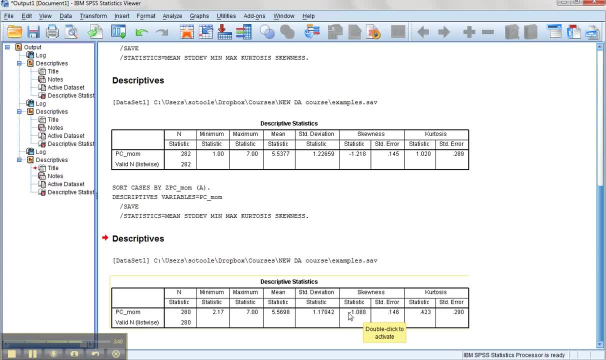 Our cartousis got a lot better. Our skewness didn't change too much, So at this point we've adjusted that variable in a relatively okay way. Another way you could have dealt with it and especially if you have outliers at both the 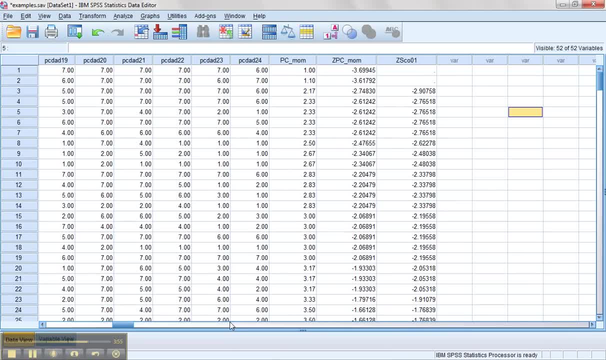 positive and the negative end, then you could have dealt with it in a relatively okay way. Another thing you can do is just come in here and hit your delete key, but make sure that you actually note what you deleted. So we deleted a value.